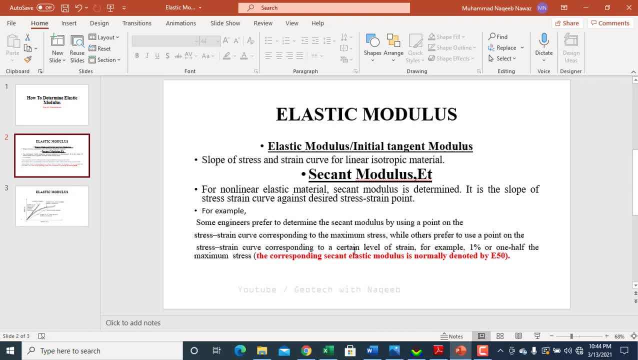 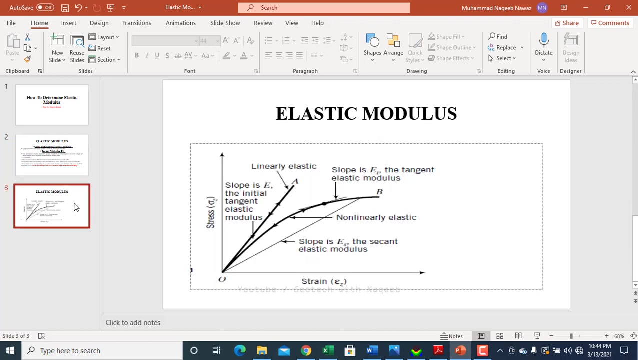 to use a point on the stress-strain curve corresponding to a certain level of strain, For example, the corresponding secant modulus is usually determined by E50.. E50 is used in numerical simulation in many of the softwares, For example in PLUXIS 2D, So it depends which. 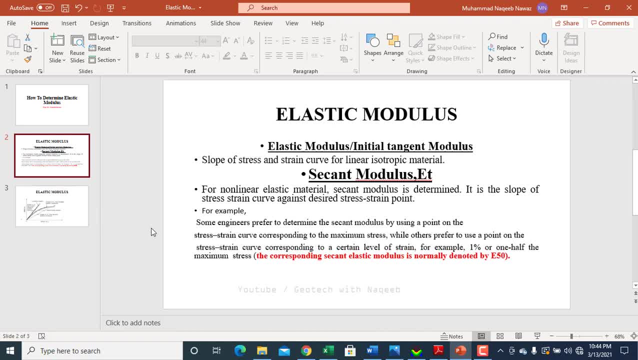 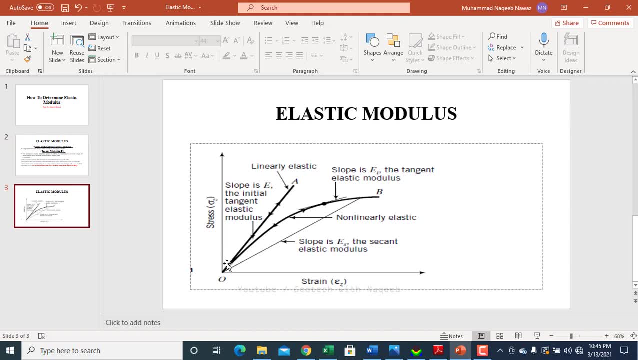 parameter you want to use for the simulation purpose. So mostly engineers prefer to use E50. so let's try to understand this concept through a graphical of this figure. from this figure you can see this is stress strain curve. so stress can be in the form of debitorics test. if we are discussing about the triaxial test, it 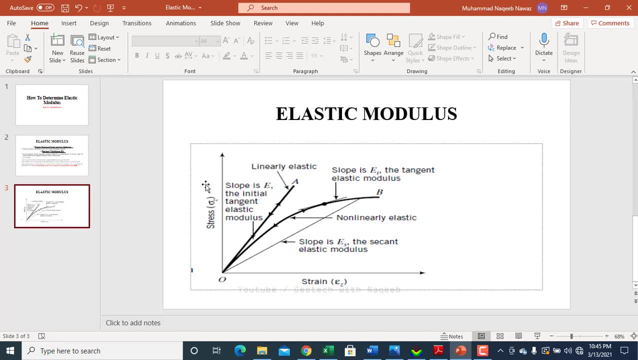 can be CD test, it can be UU test or it can be CU test. so stress is debitorics test. so this thing we have discussed in my in in our previous videos, you can check on the YouTube channel and the next thing is strain. so the strain is in. 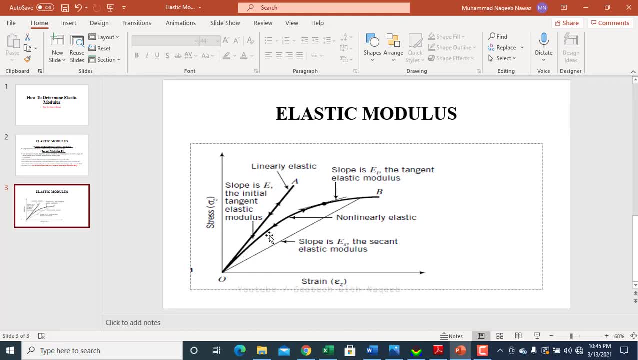 percentage. so let's say this is stress strain curve. so the initial tangent, if a slope at the initial stage of this curve- this is called the slope of this line- is basically called initial elastic model. you can see that the slope of this line is basically called initial elastic model. 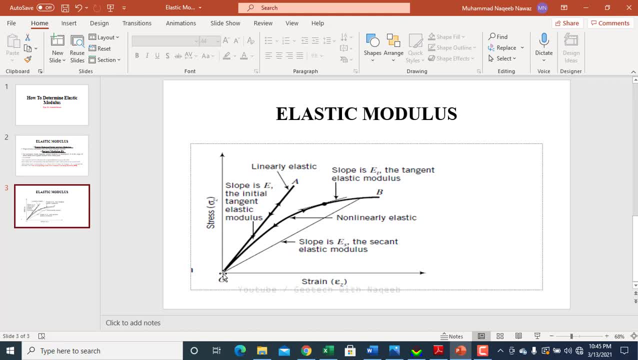 but if we want to determine the secant modulus, then it will be. it will be the point of maximum stress and corresponding strain and that slope is basically called secant modulus and the half of this is basically called E50. so let's try to understand through an example. so I have the stress strain data. 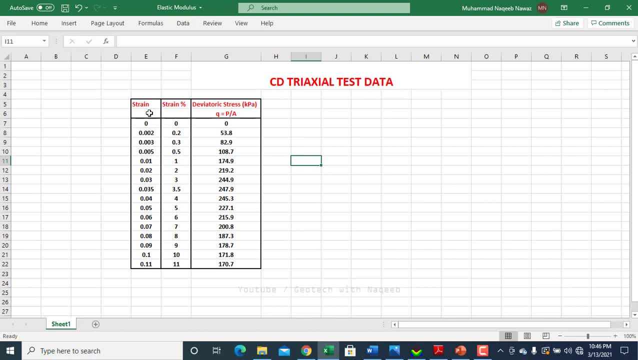 from E50. so let's try to understand through an example. so I have the stress strain data from of from CD triaxial test. this is strain value. these are strain values. while this column contains the values of debitoric stress, it can be sigma 1 minus sigma 3. 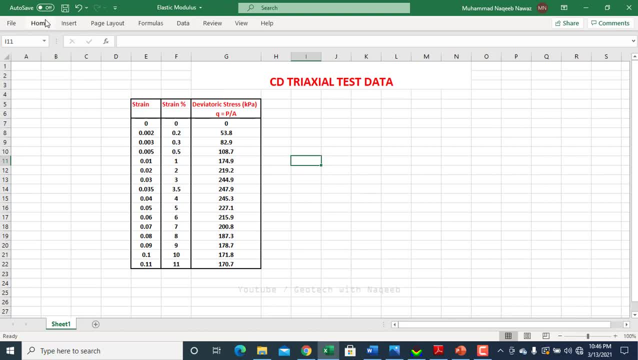 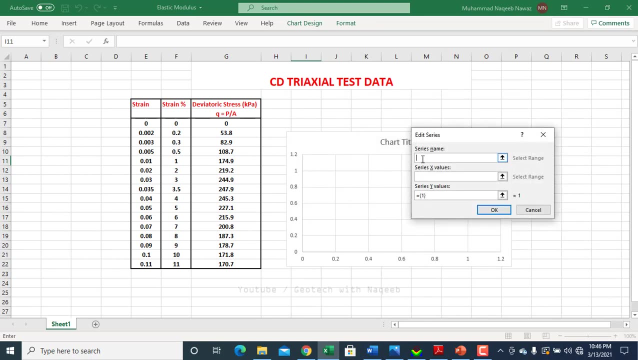 basically so. firstly, we'll draw a chart chart. we selecting this scatter chart, then right click and select data chart. then right click and select data. here you're writing stress strain. here you're writing stress strain along x-axis. I'll be plotting percentage strain along x-axis. I'll be plotting percentage strain. 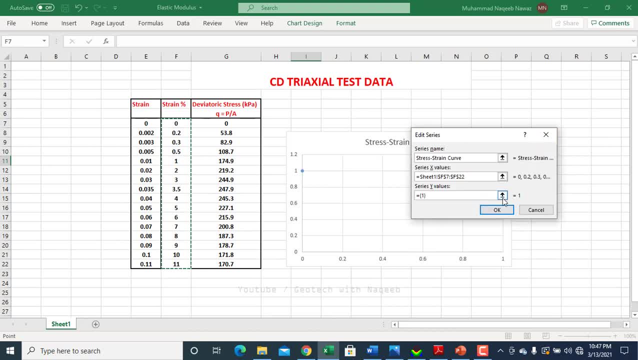 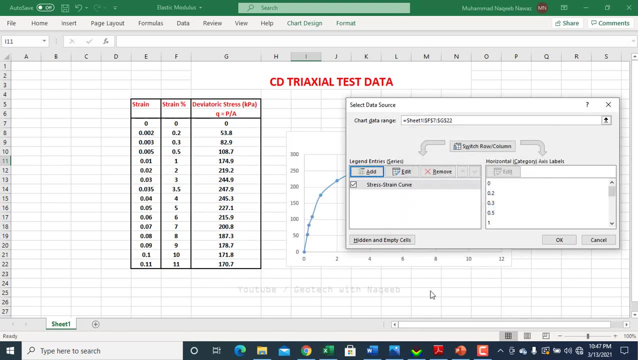 you can plot this: strain values as it is, and then, and then stress value, or debitoric stress value or debitoric stress along the y axis. so this so we tool of staying, stress value of the vector stress along the y axis. so this so we tool of things. so we will obtain this million 하고, so we can obtain these many, nogle很多. 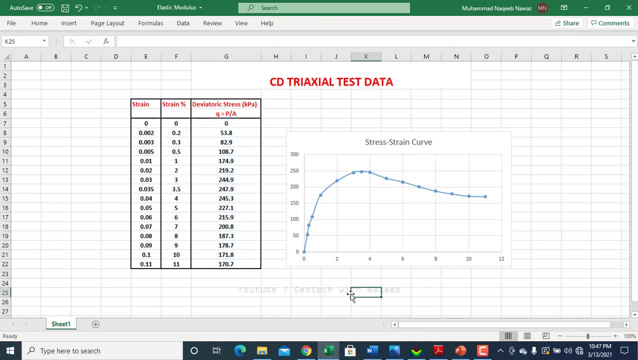 です, and then stress value. so we will obtain this millionród translated from the reading of this comparison, this stress strain graph. Now I want to determine the elastic modulus. Firstly, I will be determining the secant modulus. So secant modulus is the slope of the, or it can be the point of. 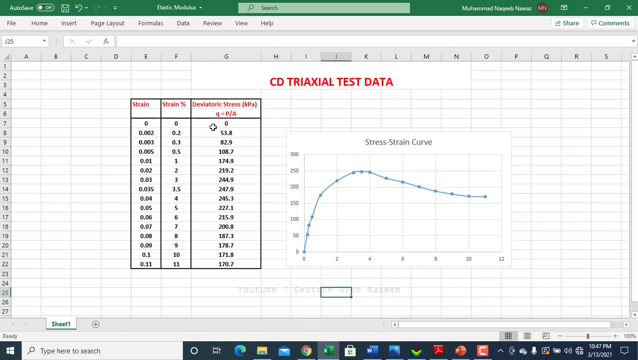 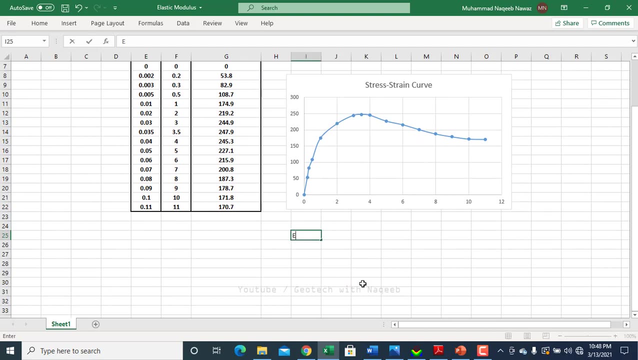 maximum stress and corresponding. So you can also observe the maximum stress point from here. and the maximum value is 247.9 and the corresponding strain is 0.035.. So you can simply find out E value by simply. you can apply the formula of max, you can you. 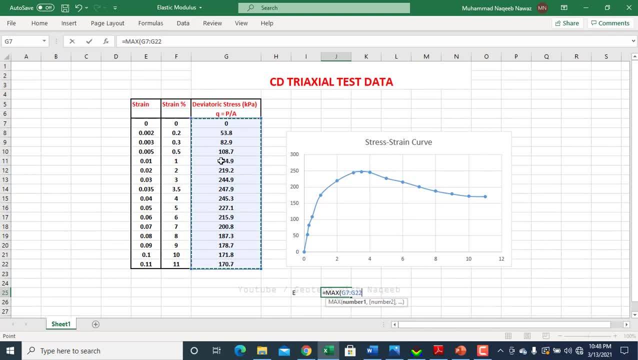 can extract the maximum value from the column of this debitoric stress by simply applying the formula of max, then close and divide it by the corresponding strain. So as we know that the maximum stress value is 247.9 and the corresponding strain value is 0.035.. So 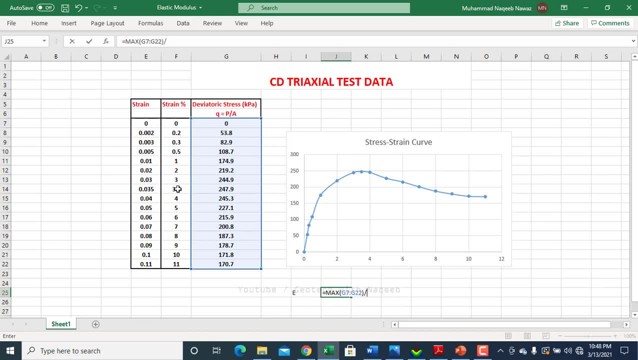 remember, you will not take the percent values 3.5, you will have to take the original value, that is, 0.03035.. So I will be selecting this column as 0.035.. So, remember, you will not count it as 0.035.. So, depending on the value, as we with respect to the time, claim, lesion length of the storm is taken from the column, and this value is secant modulus in kPa. So this is how we can find out the elastic modulus of the soil form. triaxial test data. You will find the initial tine or initial secant modulus For this purpose.